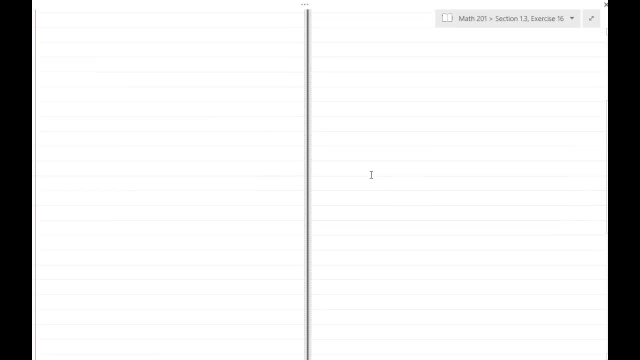 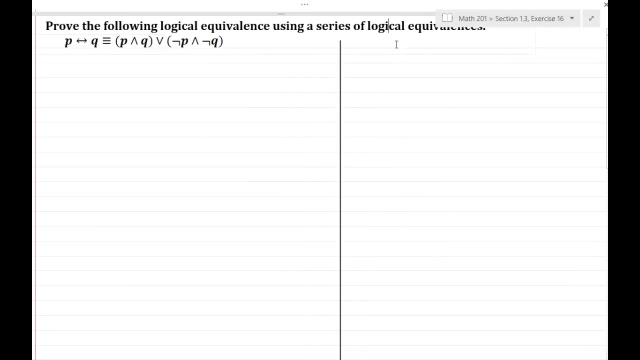 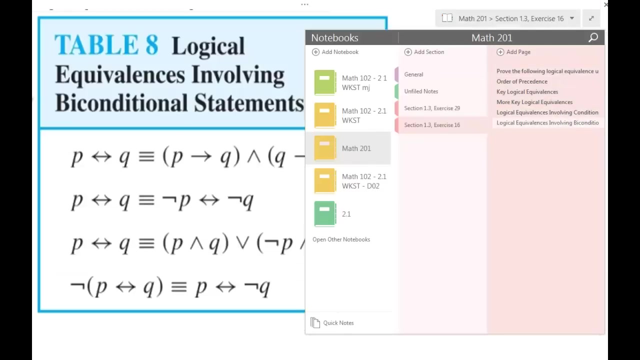 it's going to take some time and practice to wrap your head around this process and just stay patient with it and you'll be okay. So what we're doing is trying to show P if, and only if, Q is logically equivalent to P and Q, or not P and not Q, And so, if you notice here this is listed in the table with logical equivalences involving biconditional statements. 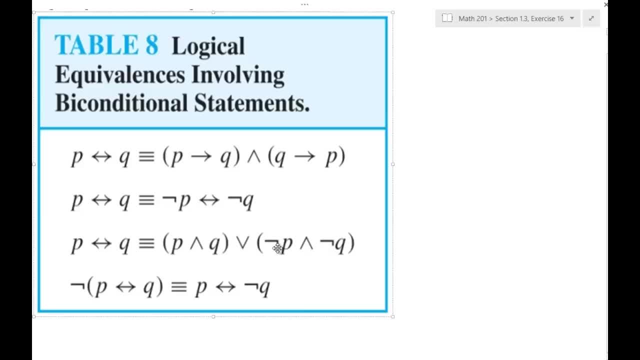 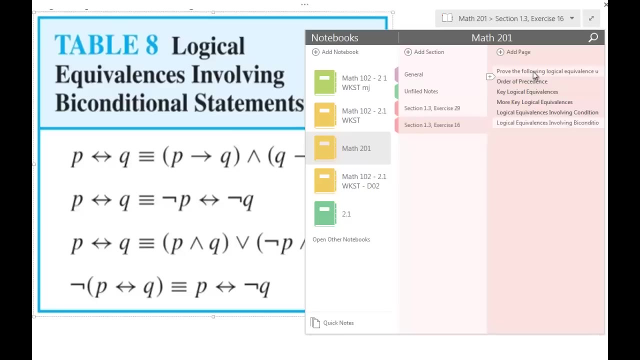 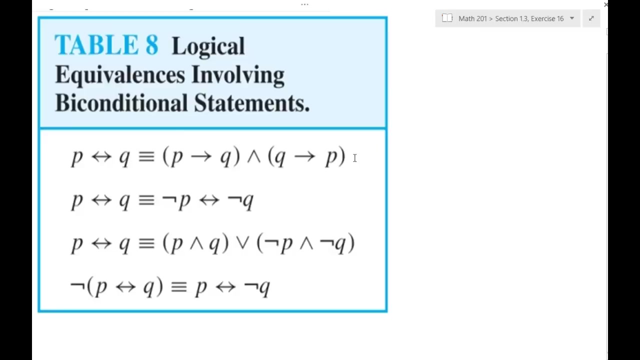 You can't say: see table eight. This proves logical equivalence. That's silly, That doesn't make sense. It's like saying, well, that's the way it is right, It is the way that it is. That doesn't make sense. So we're going to prove it with with all the other logical equivalences that we know And, just like the last example, our working goal is try to get all ands and nots and see what that gets us And always keep in mind where you're trying to go, Remember, and also the way you're trying to go. 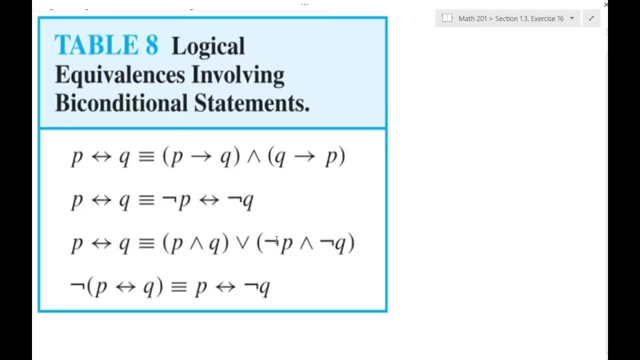 Where we're trying to end up has all ands and ors and negations. So that's not that odd of a goal here to try to get all ands and ors. And what I'm noticing with the implication is it'd be nice to write it, or the biconditional right, It'd be nice to write it as two implications, And then I can write the implication as ands and ors and kind of get on a path there. So I know for sure I'm going to use this first logical equivalence from this table. 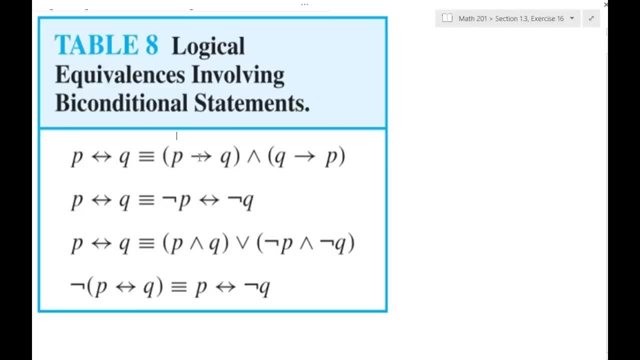 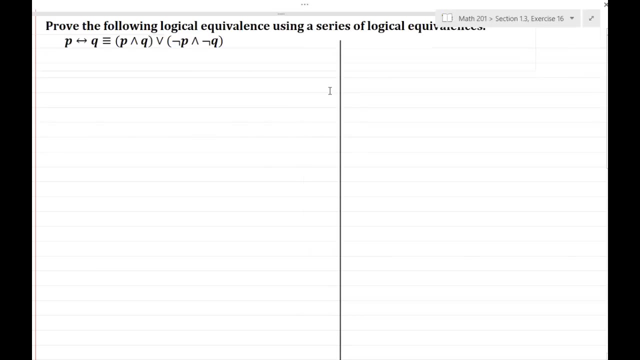 And then from there I'm going to think about P implies Q being negation of P or Q and apply that here and just see where that gets us. Hopefully somewhere right. So let's get started. How do you know which side to start on? That's tricky. You could start on either side, okay, It'd be interesting if anybody wants to write up starting on the right hand side and show this logical equivalence. 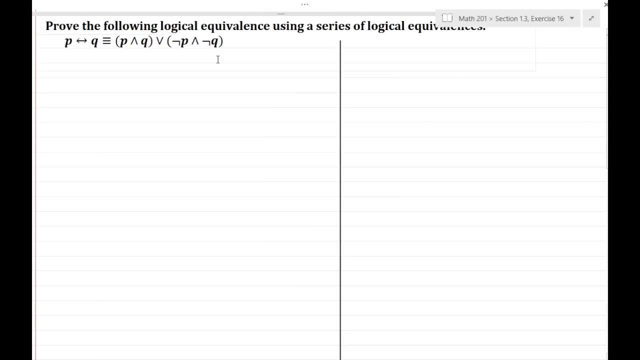 So you can get five bonus points for the week. I think that's fair to go in that quiz and quiz section of your grades. But I'm going to start with the left hand side and prove the logical equivalence. So I'm going to start with P, if, and only if Q. And you know what? I don't even know why I want to start there so bad, but it just seems like a good place to start to me. So I'm going to start with the P, if, and only if, Q. 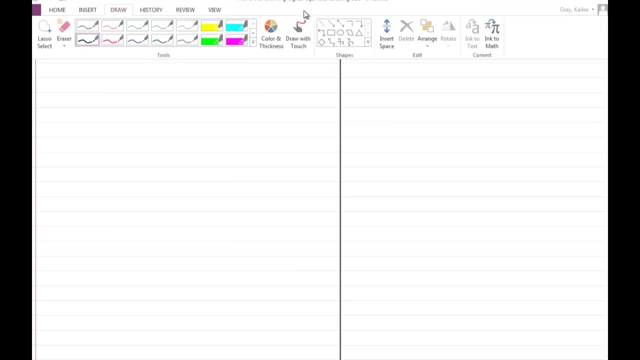 And I don't know, probably, like I said before, if you've taken trig, you've dealt with proving trig identities, So you might, you know, kind of get a feel of remembering that experience. And so one thing I thought in trig was that we'd always start with the more complicated side, but I don't know if that's necessarily true. It's just kind of start somewhere and see what happens. If you're not getting anywhere, then try the other side. Okay, so I don't think there's a hard rule for that, But remember you can only work with the right hand side. 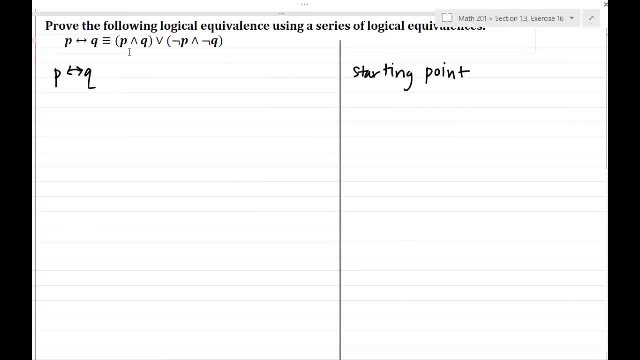 You can only work on one side at a time, Okay. otherwise you're assuming the equivalence and we don't know the equivalence yet. So we can only work on one side of this at a time, Okay. so we're only going to work with P, if, and only if, Q. So, like I mentioned from that truth, those logical equivalence involving biconditionals, I know that a biconditional is just two conditionals going in each way. So P implies Q and Q implies P. So I'm going to start here with this logical equivalence. 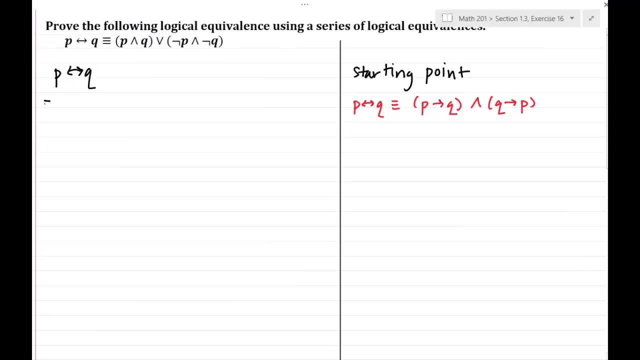 And I'm going to rewrite my biconditional in its equivalent conditional form. Notice I'm only substituting with things that are actually logically equivalent. Otherwise it doesn't make sense. And I've got a justification for every single step And it's very clear, and it will be very clear in your work why you're doing each step. So really work on this idea. I think it'll help us both be more effective. I'll be more effective in grading and you'll be more effective in the grading. 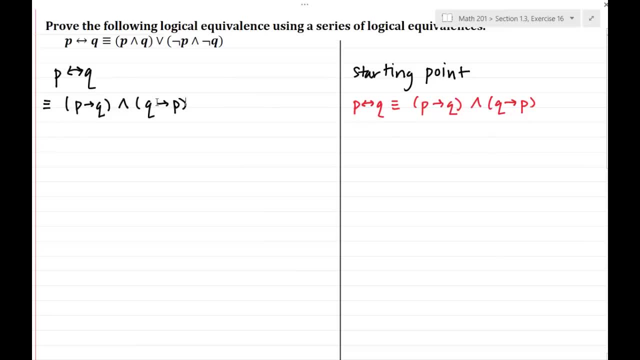 This process. So so now again, I want to try to get all ands and ors Okay. so what I'm going to do next is just use that logical equivalence with the conditional. I know that the hypothesis implies the conclusion is logically equivalent to the negation of the hypothesis or the conclusion. So what I'm going to do is go ahead and replace both of these implications with their equivalent negation or form, And I you know there might be words for this or whatever, but I usually don't. 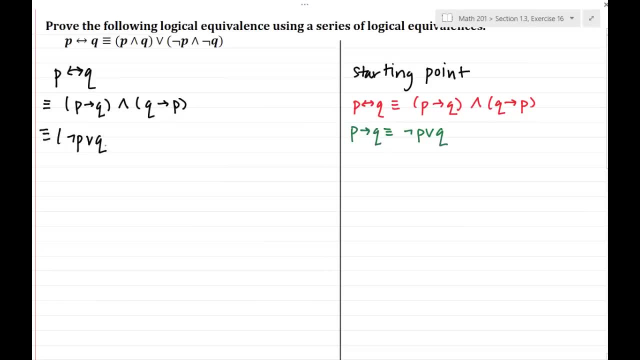 just say, you know, negation or or whatever you want to say. But but when you're justifying, just write out that equivalence that you're using. Don't worry about the, the words and and names for now. Just write out the logical equivalence that you're applying at each step. So P implies Q is logically equivalent to negation of P or Q. Again, I think of hypothesis implies conclusion: Negation of hypothesis or conclusion. Hypothesis is Q. Conclusion is P: Negation of hypothesis or conclusion. 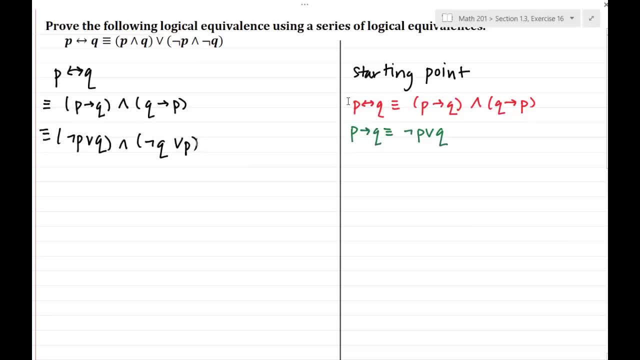 Hypothesis would be negation of Q or P. Okay, don't get caught up in these P's and Q's. Okay, they're going to trip you up. So just think you know. first, second hypothesis, conclusion, right, And remember, with the implication, the order is important, Okay, so it's really important that you negate just the hypothesis, right, And you don't switch those around. All right, so now we got something to work with, But what are we going to do with it, Right? Okay, let's. 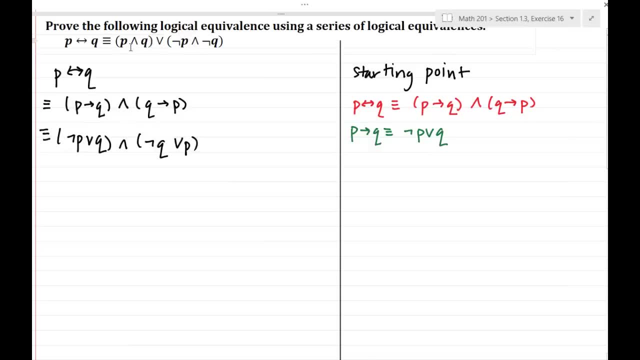 let's think about where we're trying to go here. I know I want to put the P with the Q right, And now I they're kind of separated right, These two ors are grouped and kind of separated, And I'd like to have the P by the not P. That might help me, But but I would also like the not Q to be by the not P, So somehow I need to combine these guys, Okay, And the way I'm going to do that is is try to think about this first one as just one thing, Kind of think about it like M. Let me put this to the left. 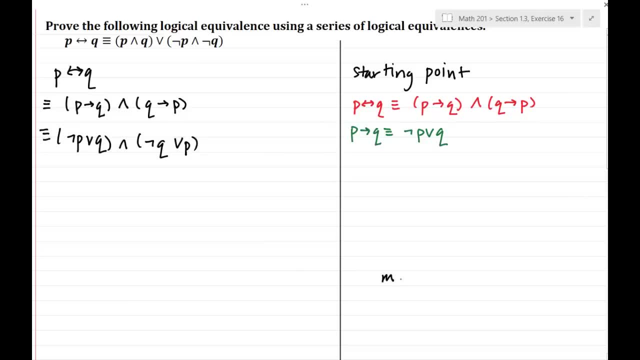 Kind of think of it just like some proposition M, If we've got M and not Q or P, we could use distribution here and write: you know, bring that M, not with you and, or the middle M and with you, put, or in the middle, So M and not Q, or M and P, Okay. So so think on that And see if you see what I'm doing. 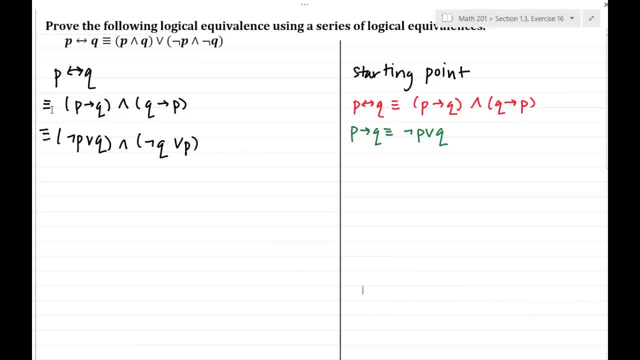 See what I'm trying to say here. I think what I'll do, guys, is put in a little quiz here for the correct distribution of- well, I've got to write this down: The correct distribution of not P and not P or Q over not Q or P. Okay, So pause to do that quiz. 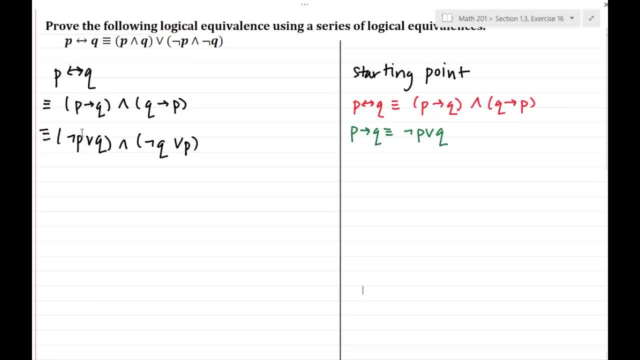 All right, Hopefully you did that And it made sense. And so now let's think about this. I'm going to use distribution. P and Q or R is logically equivalent to P and Q or P and R, So I took that P and put it on the Q. 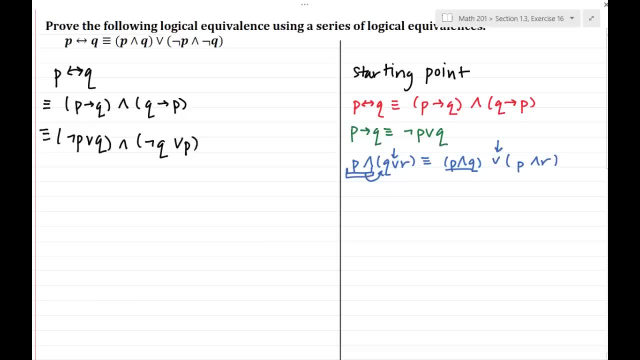 Separated it by an, or Took that P and put it on the R. Okay, Notice, you can distribute from the right or the left, It doesn't matter, as long as you do it correctly. Okay, So I'm going to take not P or Q. 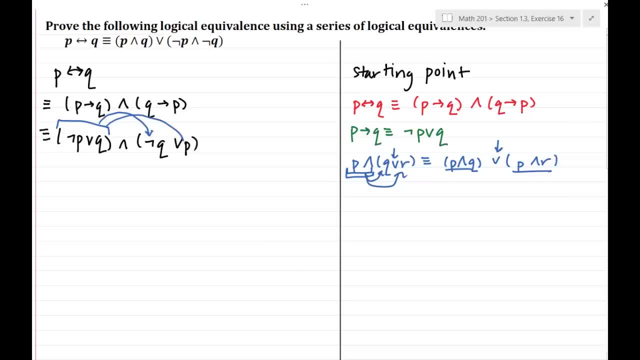 Apply it to, not Q, And apply it to P, Put an or between: Okay, So let's write that out, See what happens. So now this is tricky right, Because I don't just have P, I have a compound proposition going on. 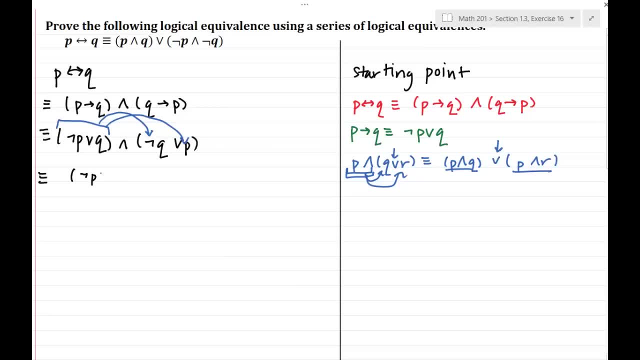 So just be really careful, Make sure you group things appropriately And don't lose any parentheses. Okay, And not Q. All right, That's grouped. That's grouped. Or. And we're going to distribute the, not P or Q. 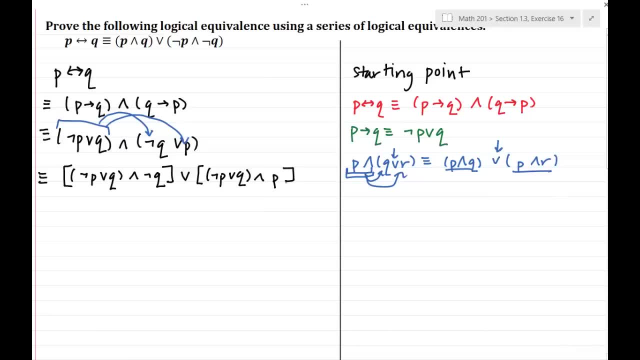 And P. Okay, Now this is looking like something we can work with a little bit better, Because now I notice, oh, I've got this negation of Q a little bit closer, The negation of P, So that's nice. 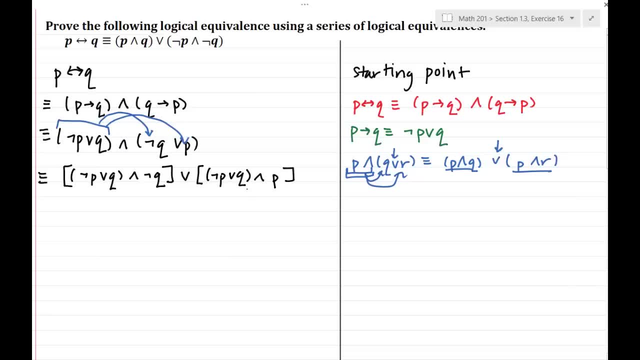 And I've got the P closer to the Q, So we are moving in a direction that's good. Okay, Now notice how we've got a bunch of different operations going on. Well, we have a bunch of and and ors, And that's tricky to work with. 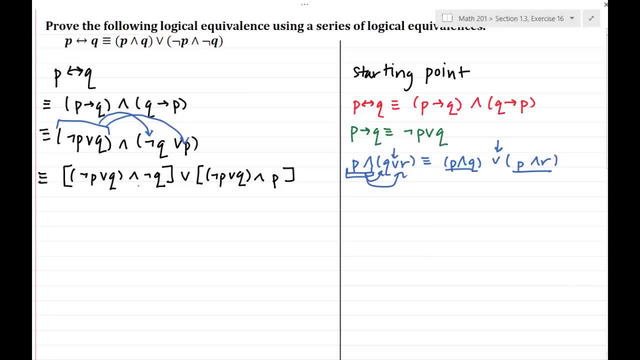 Because we can't really move things around in a way that we want to necessarily. So if we could get all ors or all ands or something, that would be wonderful. Probably not going to happen, right? Well, definitely not going to happen. 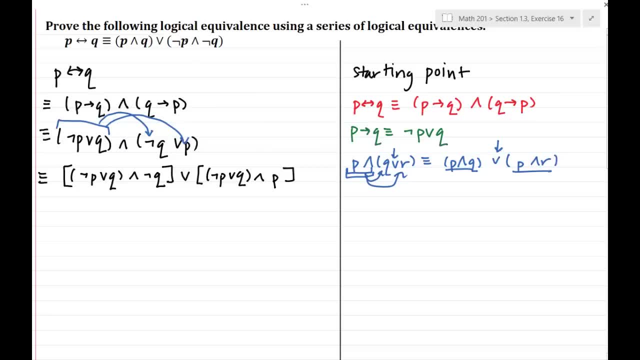 Because look at our final product. We should have ands and ors going on. But- and maybe that's not the best argument for this step- Maybe the best argument for this step is just what I said before, That I want to get not Q by not P. 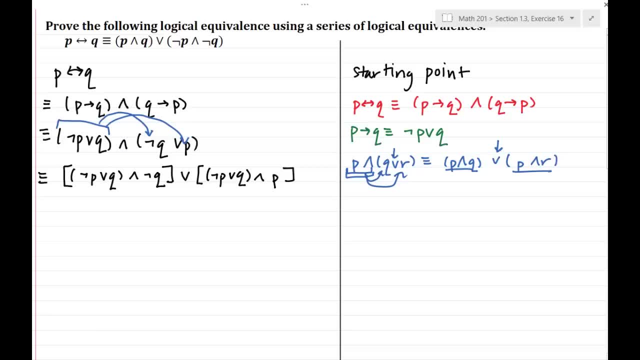 And I want to get P by not P Or P by Q right From here. So I'm just going to use distribution again. What I'm going to do is: let's see The form that I've got. going on is an or. 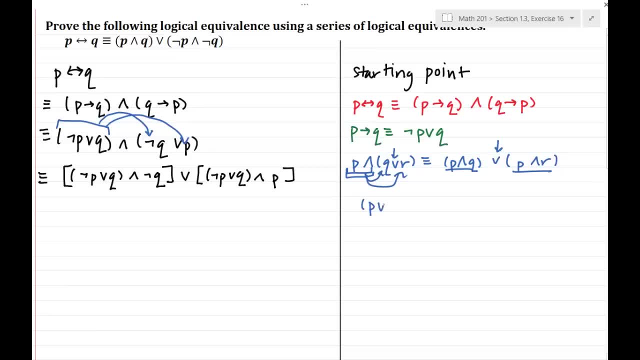 Which is actually the same as the one I wrote, But it's just a different order. But it still works in the same: P or Q and R is logically equivalent to P and R or Q and R. And you know, even though symbols change the operation and their order and the way that they're grouped, 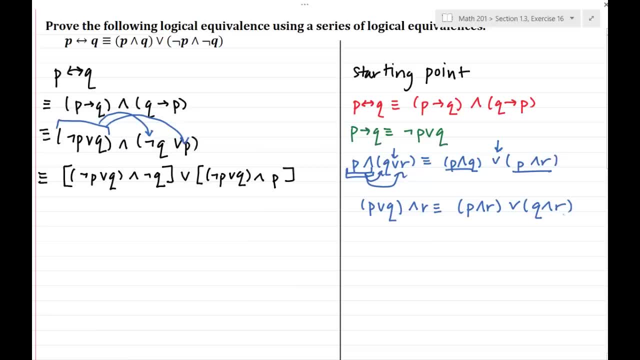 it stays the same, so that the principle still applies. Okay, hopefully that makes sense, Because be careful here. This, this statement here, is totally different from this right. The P and Q do not overlap. Okay, It's just two. 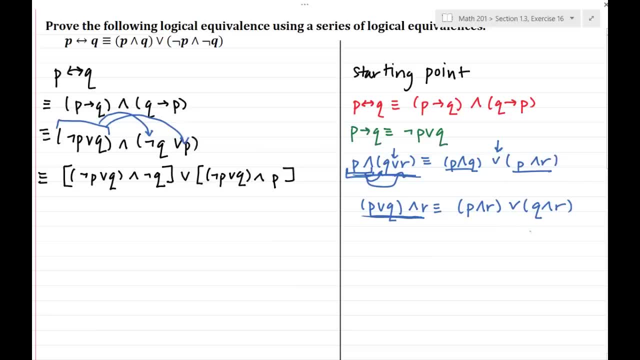 Two different ways of stating the distribution process, property, Like, like. if I that distribution of five, example two plus four times five, I can use the same principle with five times two plus four, right, In that case? you know, our, our meaning is the same. 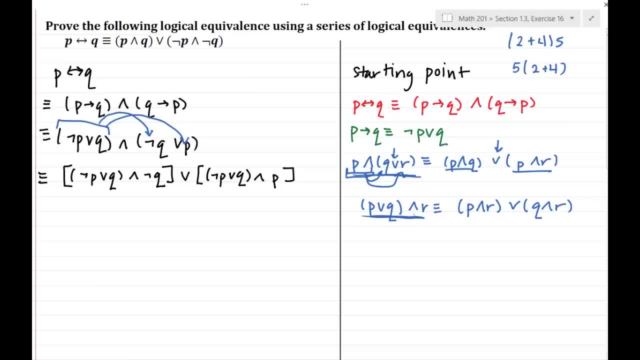 But this here a little bit different. Yeah Well, because I've changed the order of my variables. But ah, that's still what we're. So what I'm going to do is distribute the not Q to the Q and to the not P. 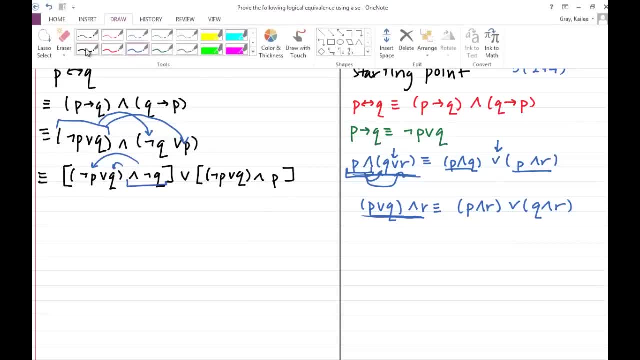 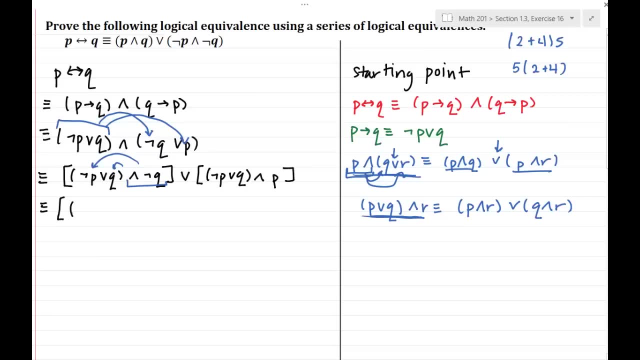 And I'll put an or in the middle, So I'll have again. I'm going to make sure to group this so I don't get things combined with other things. You know, if you're trying to err on the side, try to err on the side. 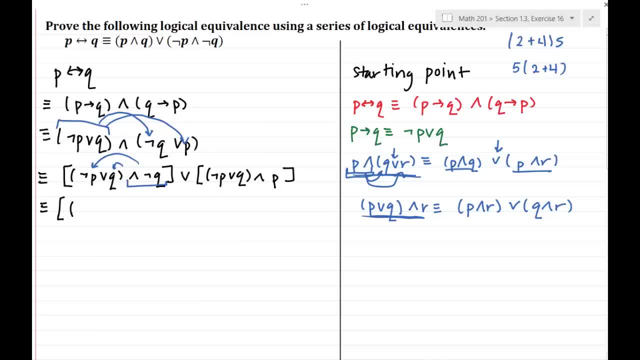 of putting too many parentheses in, okay, So as long as they kind of make sense there, Just be careful. Yeah, be careful, Not P. Okay, I'm distributing the not Q to both of those Now putting an or between Q and not Q, All right. 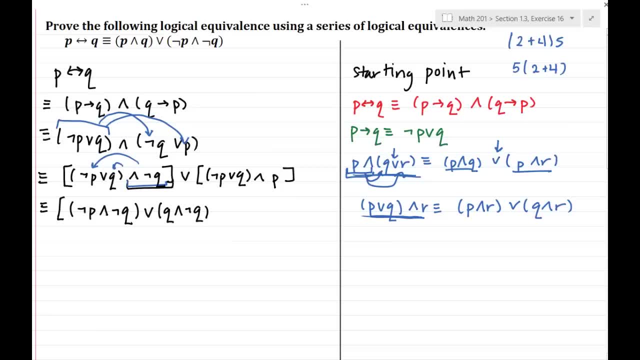 So what did I do? I took the, not Q, the and not Q, wrote it after the not P, So not P and not Q, Split it up with an or And, then applied that and And not Q to Q. 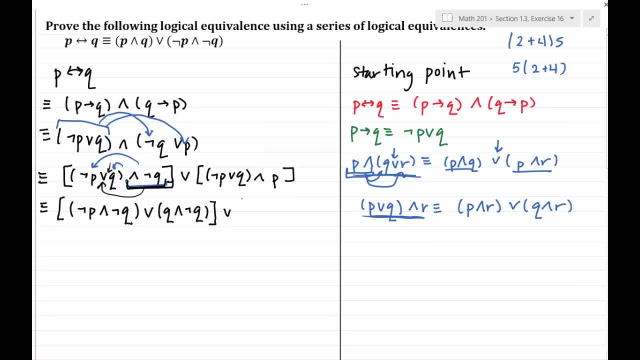 So hopefully that makes sense there, And I'm just going to focus on that little piece for now. I could do that with the second one, but let's not bite off more than this one step. okay, One step at a time, all right. 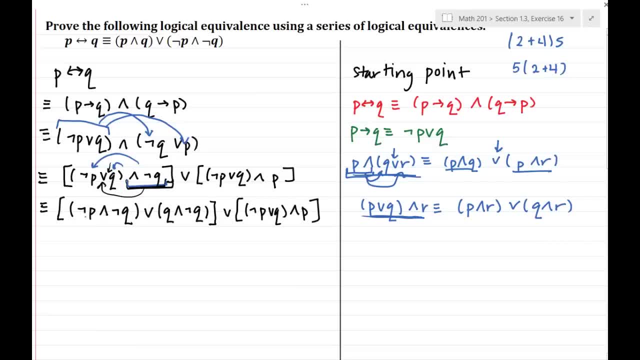 Okay, Now it's looking kind of nice right. I've got that- not P and not Q, which is where I want to have well, what I want to have right. So I like that, this Q and not Q I don't like so much. 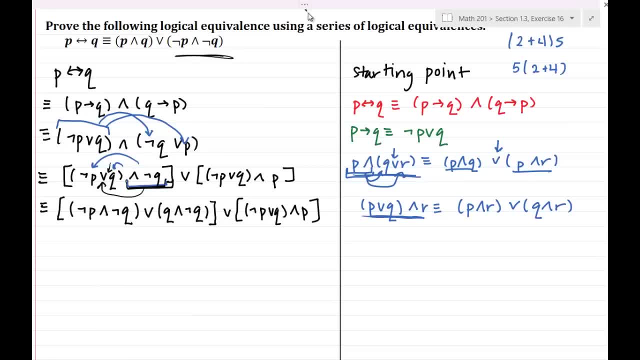 Let's think about that. What do we know about a statement and its negation joined by and? And let's do a quiz: What do we know? Answer would be like a multiple choice thing. okay, And I might just link these all in the same quiz, okay. 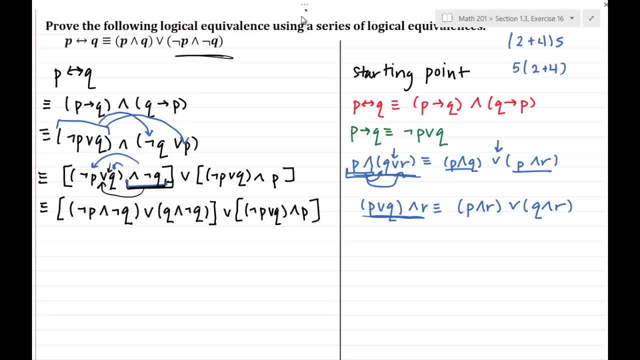 That might make more sense. So go ahead and tell me. What do we know about a proposition joined by It's negation with and? Okay, and I'll give you some multiple choice there, okay, So let's see here. 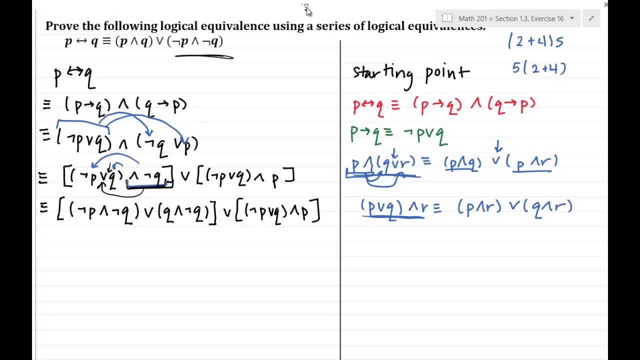 So the answer which hopefully you did on the quiz and you're not just watching. okay, Take a moment, It's for your own good to think a little bit. Hey, come on guys. All right, So what we're going to use here? we're going to use the fact that, if I take a statement, 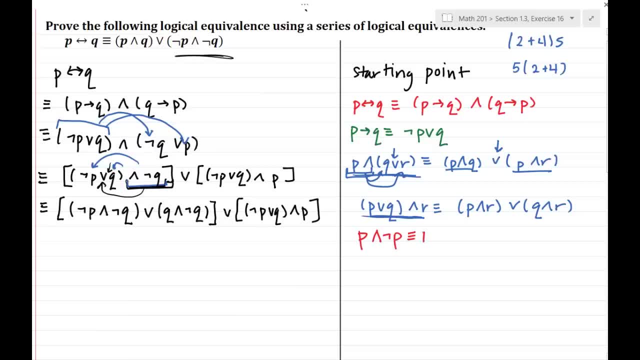 and its negation. it's always going to be false, Because- and both of them have to be true, with and But- if I have a statement, it's a negation. They're always going to have opposite truth values, So it's always going to be false. 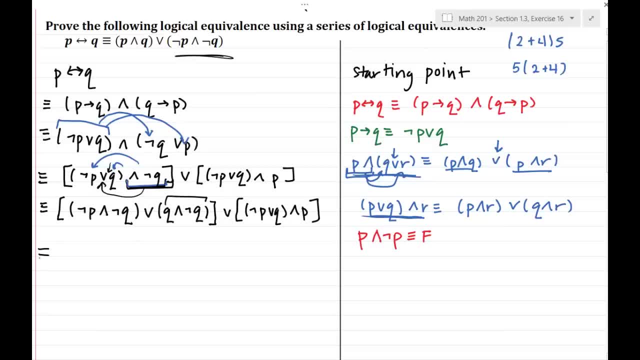 So I know that Q and not Q. that's false. So I still have my not P and not Q. I really like, because I want to see that in my final answer here, For and we're still kind of leaving this piece hanging here- 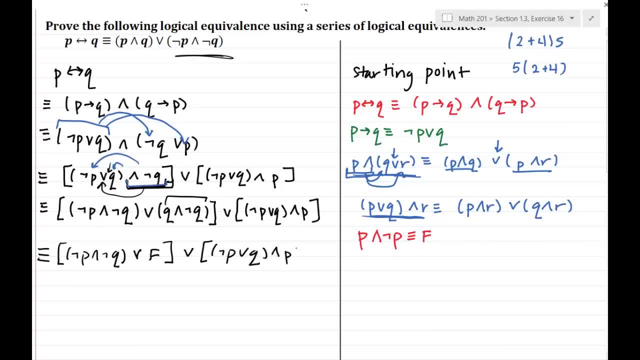 We're going to take care of it later. All right Now. what do we know about a statement joined by or to a false proposition? So my question is: what do we know about P or false? Take a moment, Answer that question on the quiz. 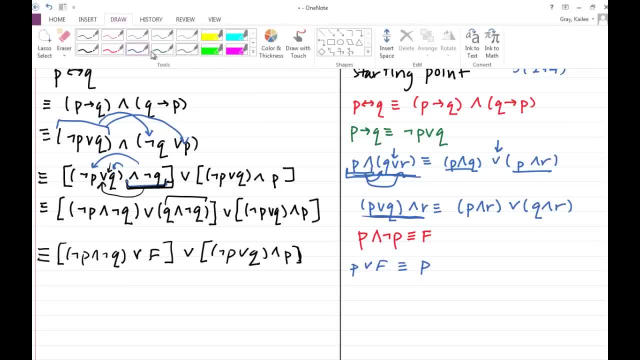 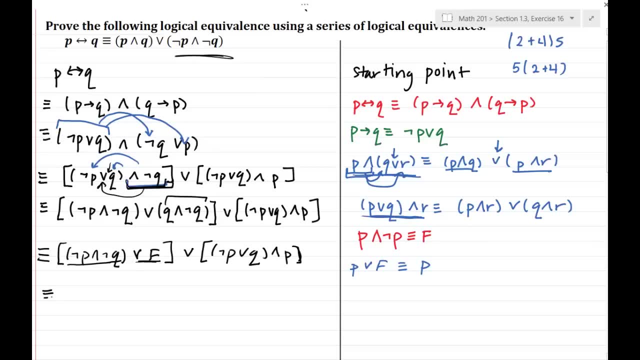 It's P, Okay, All right. So we've got a proposition, a compound proposition, joined with or with false. So that means I'll just have that compound proposition left. It's going to take over. Its truth value will determine the truth value, because we've got or. 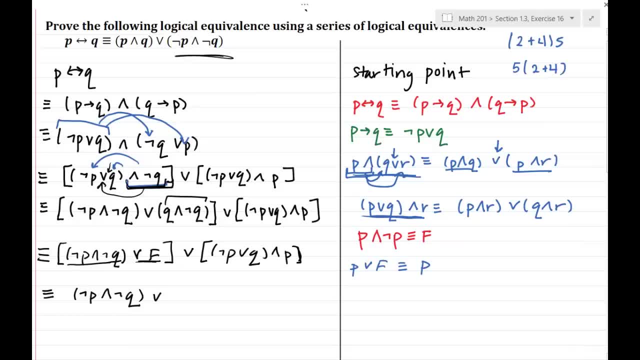 So if P is true, the proposition will be true. If it's false, the proposition will be false. So if the false doesn't affect it, it's just going to take over there, All right. So we like the way that first one's looking, because it's got this exactly. 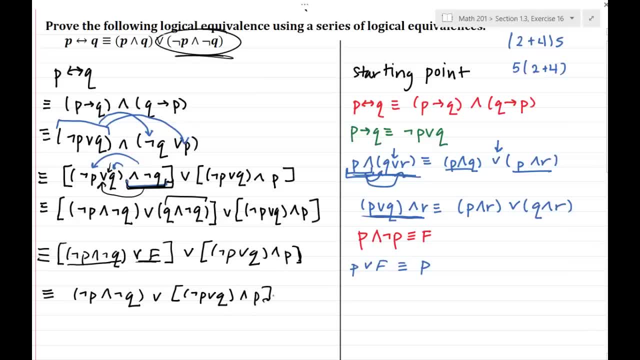 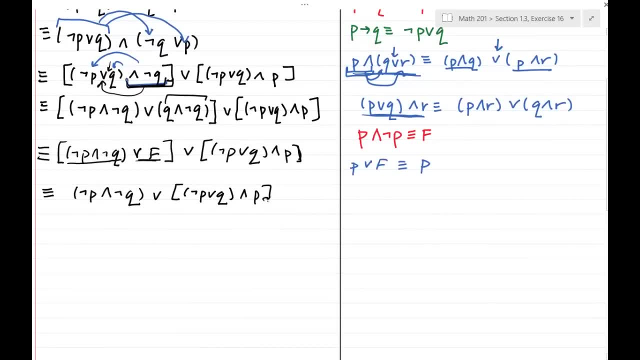 So we want to try to make this second one look like the left-hand side. okay, And this is going awfully smooth, okay, I promise you when you do it, it will not go smooth the first time, okay, And 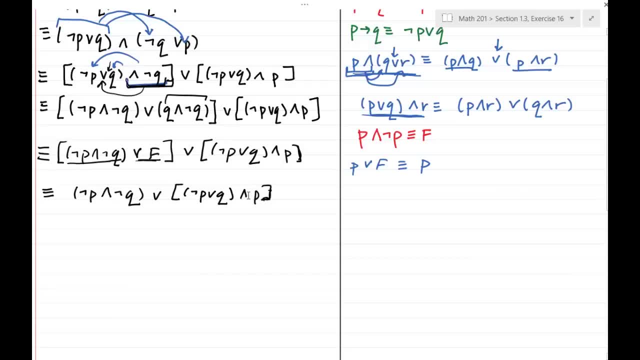 Believe me, I just learned this. you know, I don't know. Well, I don't know When I learned it. it took me a while, okay. Lots of torn up pieces of paper and frustration, okay. So this is all magic now. 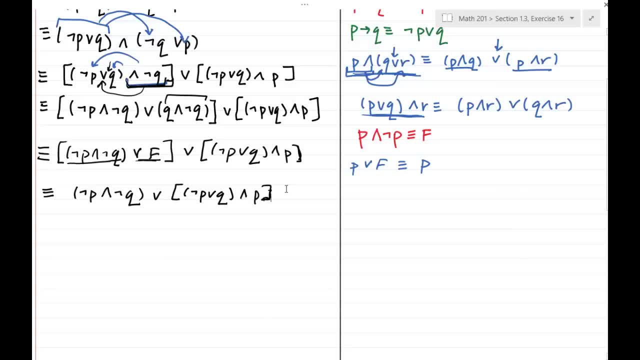 Somehow magically, I know, step to step, what to take, but you're going to have to play around and make some mistakes. okay, And that's okay. Just keep practicing, All right. So now let's use the distributive property here to combine that P with the Q. 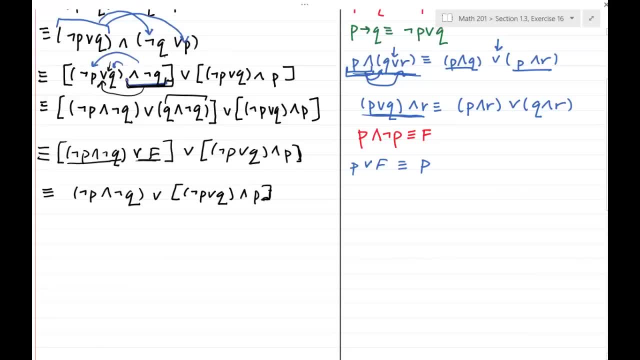 We want those guys to be by each other. So the property I'm going to use here I've got two propositions joined by OR and I'm distributing an AND R, So I've got P AND R combined by OR, Q AND R, okay. 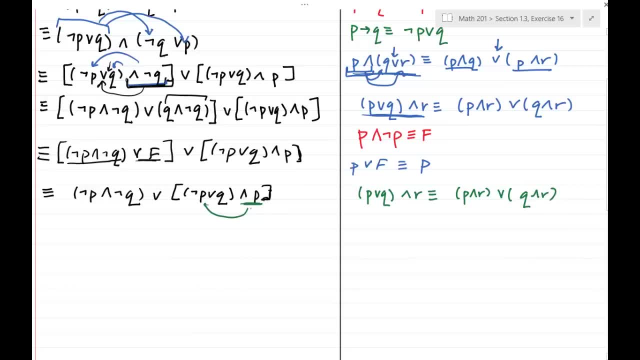 So I'm going to take AND P, distribute it to NOT P, AND P distribute it to Q, put an OR in between, And that first guy is just going to hang out for a little bit. We're not going to worry about him right now. 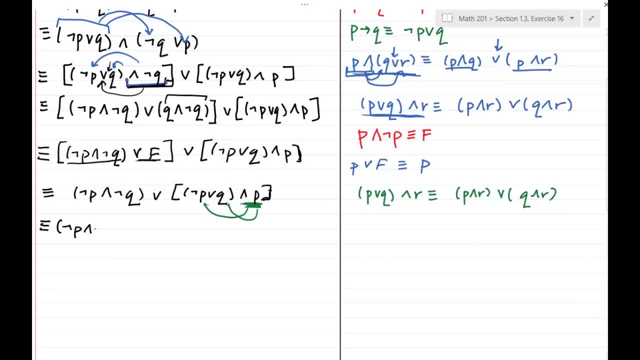 We really like him, He is looking good, He is looking good, OR and let's distribute. So we've got NOT P AND P OR Q AND P. There we go. That is looking very good, right, Because basically we'll be able just to follow these same exact steps that we did. 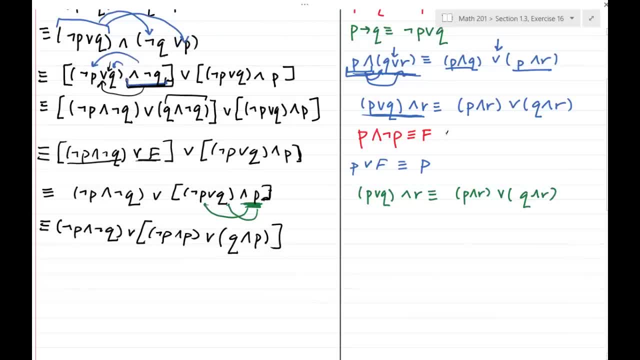 in the last one, We'll be able just to do this again: right: A proposition and its negation is false. A proposition or false, This is the proposition. So let's just apply those steps again. Let's write them down, though. 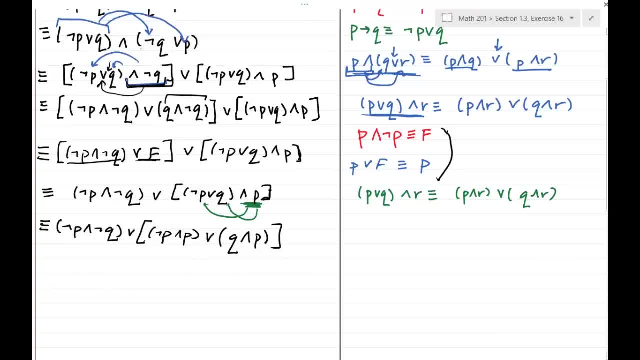 Just the way we know and your reader knows. your reader me knows what logical equivalences you're applying, Because you might think it makes perfect sense, right, But you might as well communicate it with me so that it makes perfect sense to me too. 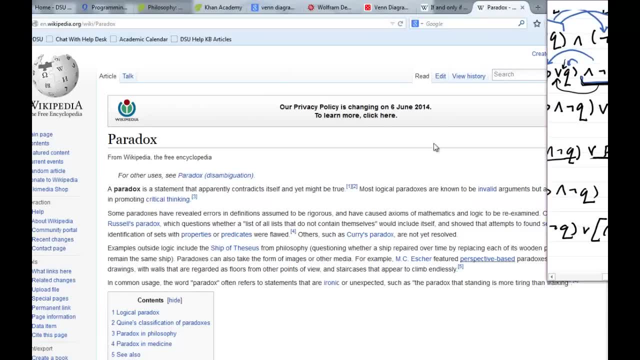 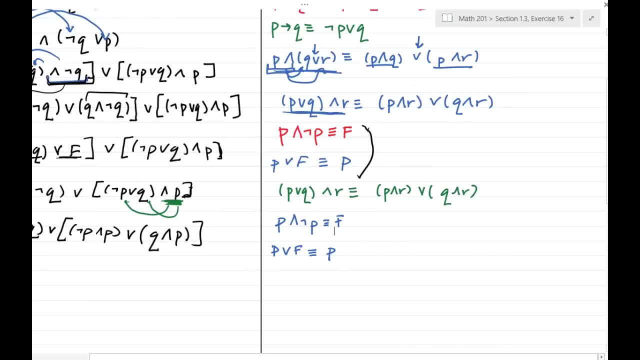 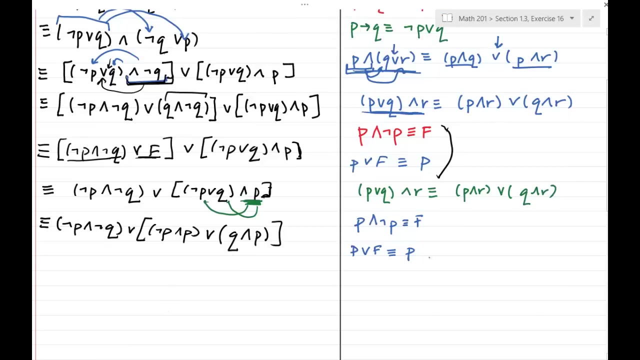 So let me in on your head. Oops, it's paradox, Oh my gosh. Oops, Hey, where'd you go? What did you do that for? Oops, Alright, So we're going to apply those properties. 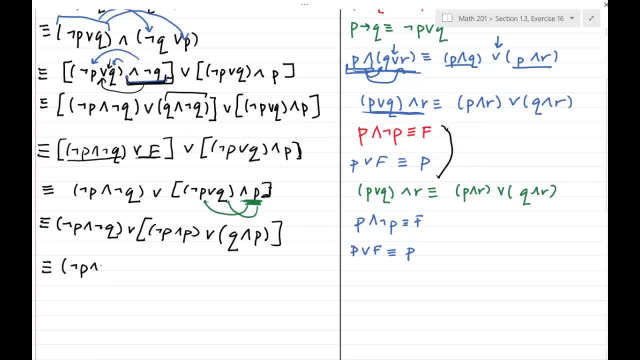 Apply those logical equivalences. The first one we're going to leave, The second one we're going to write: not P and P is false. Now, if I take false and join it with a proposition, I'm going to just get the other proposition. 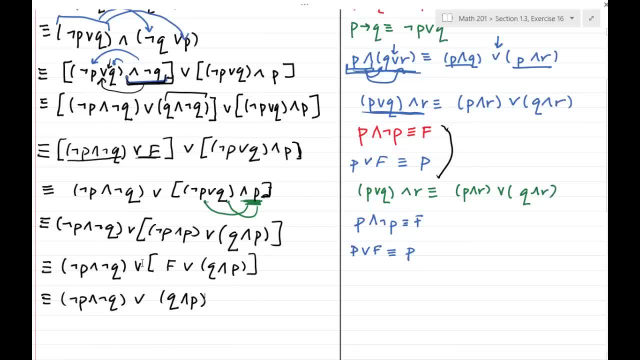 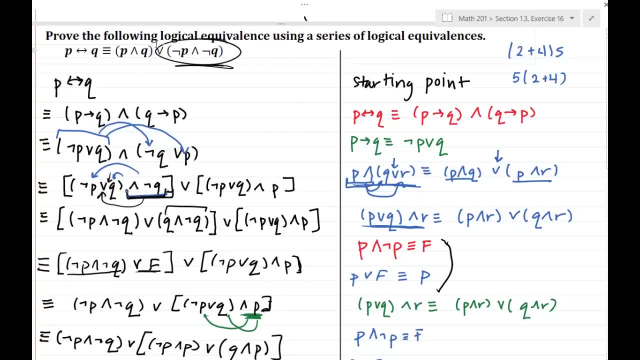 Q and P. Alright, this is looking pretty good here, Pretty good right. Here's this that we're looking for. We're also looking for P and Q, So the order's a little bit off, but we are really. 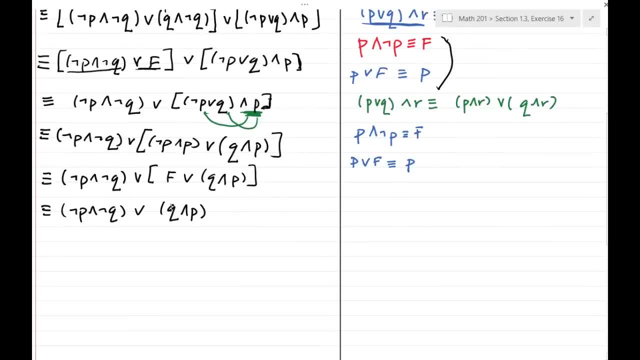 really close, so let's fix the order First, one thing at a time, okay, Don't be doing crazy, crazy things and getting me all confused. Q and P, P or Q, P and Q, Logically equivalent to Q and P. 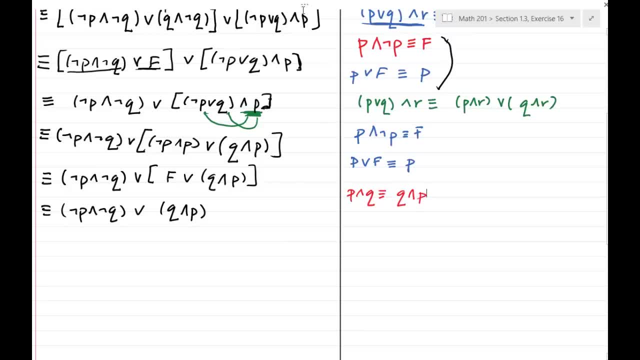 So they're commutative. That's all that. that's saying. They can be done in any order. It's just like multiplication Five times three is the same as three times five, right? So let's go ahead and apply that logical equivalence to the P, Q and P, so that that's in the order. 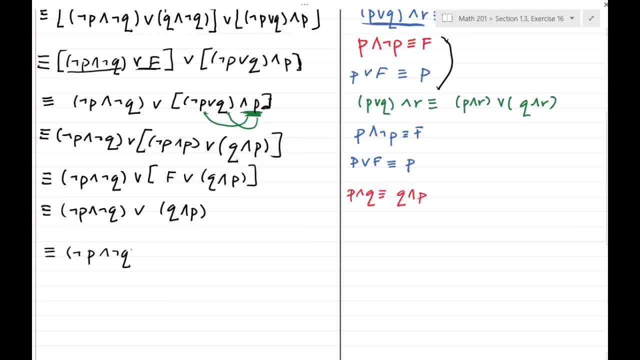 As that final compound proposition we're trying to work towards, And really I mean we should do these in two separate steps, Because I mean or list commutativity of and operator and the commutativity of the or operator. But so now we've got the innards of those two pieces in the right order. 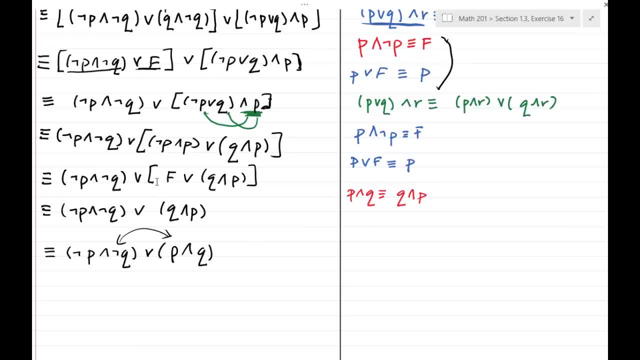 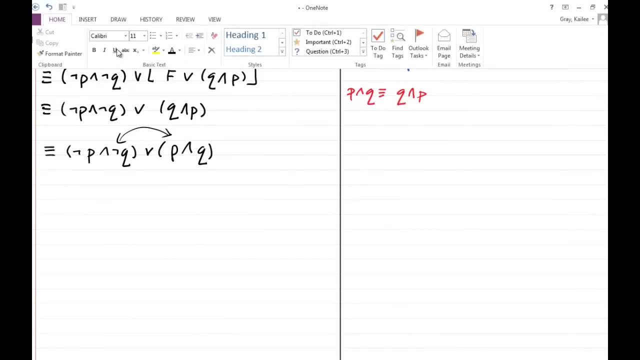 But these guys are swapped from the order of what we're trying to go towards here. Okay, We're trying to go towards this guy. So I know that or is commutative Is a commutative operation. So I'm going to use the fact that P or Q is logically equivalent to Q or P. 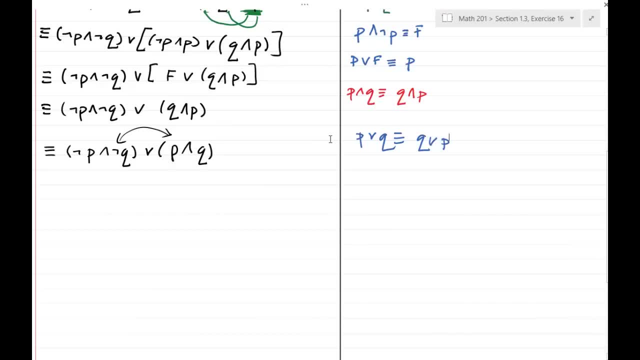 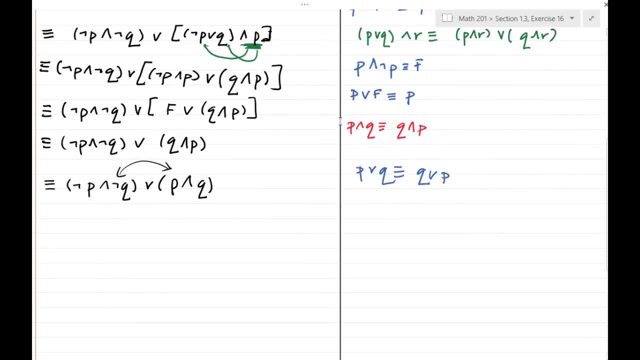 Okay, And list them over and over again. Tell me every single step, what you're doing. Okay, You might see we've written the same thing over and over again And it's annoying, but I know exactly why you did each step. 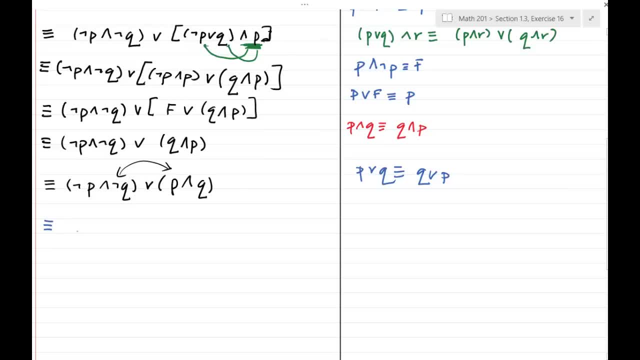 Okay, So let's go ahead and we'll have our final result here that we're trying to get to. So we use a series of logical equivalents and we replaced it And we got to our final answer. We got to our final compound proposition that we are looking for. 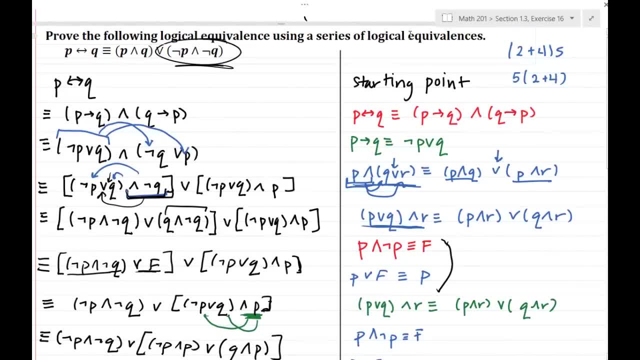 Okay, And notice the way that I stated this Using a series of logical equivalents. Okay, On your exam. Don't ignore this and give me a truth table. I will be upset. Well, I will be bummed out, You know.